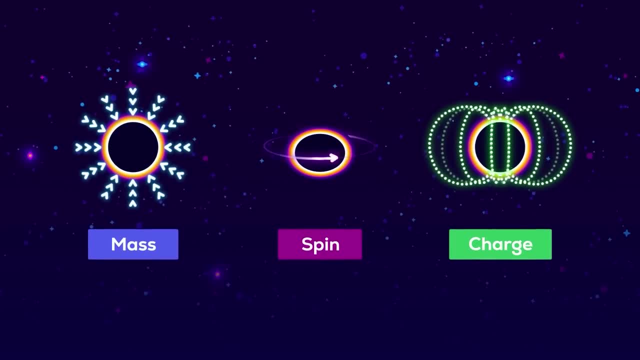 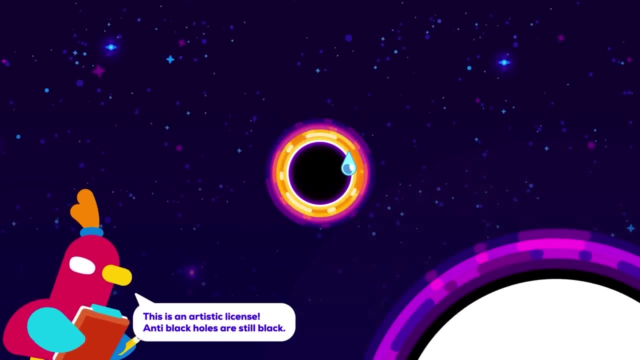 It's just a matter of how much energy it has. It will always be fully described by those three numbers, nothing else. But if a black hole is basically a weird particle, could we destroy it with an anti-black hole Experiment? 3. Anti-black. 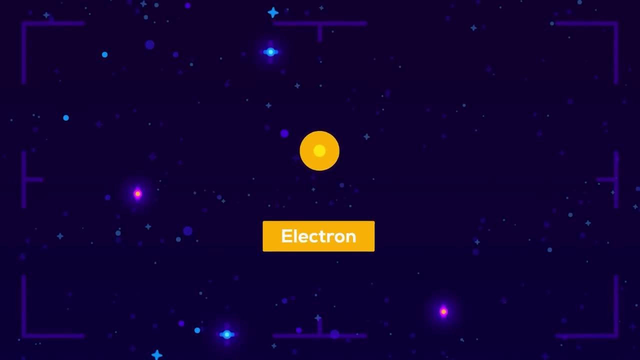 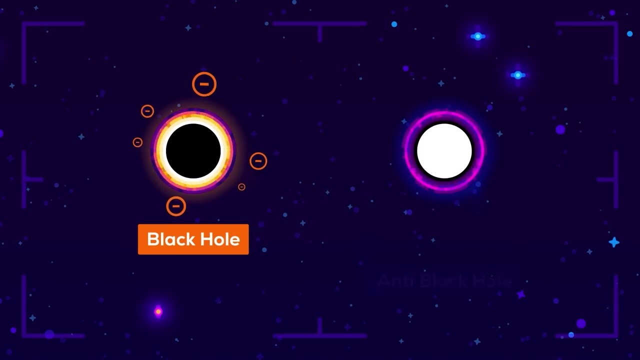 hole. How exciting. A particle has the same mass as its corresponding antiparticle, but opposite charge. Since a black hole has mass and electric charge, its corresponding anti-black hole should have the same mass and opposite electric charge. What if we make them? 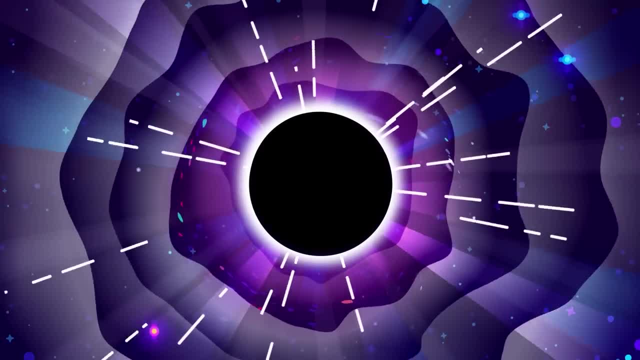 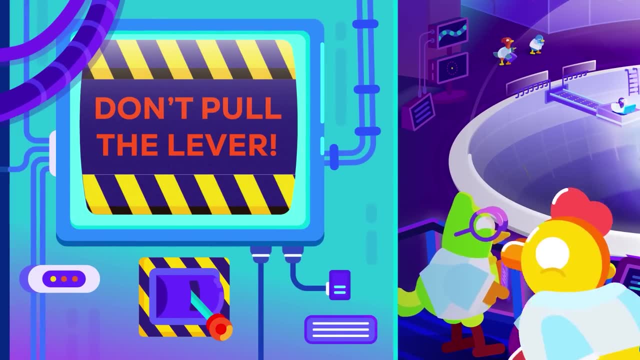 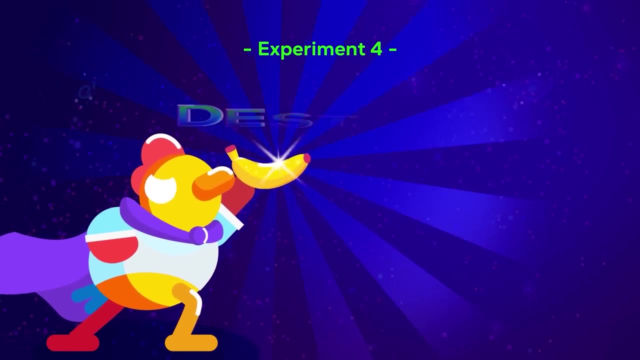 collide, Sadly, the charge will just add up and cancel out. So after the collision we'll just get a new black hole twice as massive with no charge. Okay, we need to think bigger and stretch physics harder. Experiment 4. Destroy the event horizon. It's true that a black hole can carry. 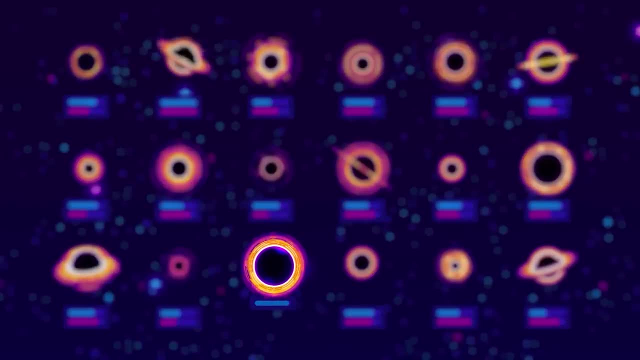 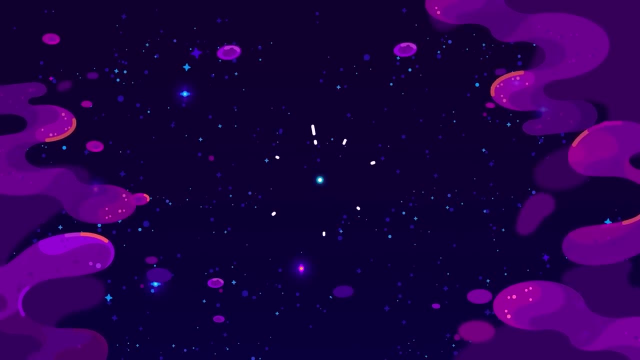 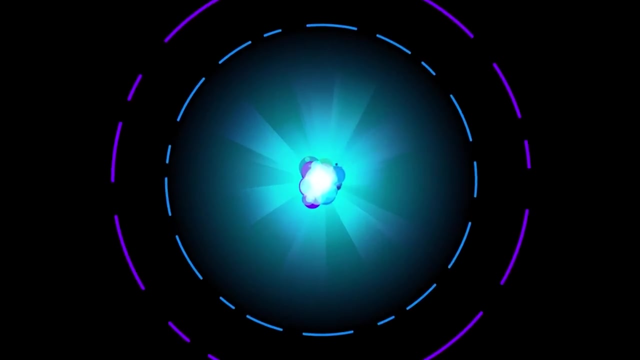 spin and charge, but even for these crazy objects there are limits. If the spin or the charge of a particle happens, the event horizon will dissolve In a simplified way. we think of black holes as hiding a singularity inside an infinitely compressed mass with such strong gravity that 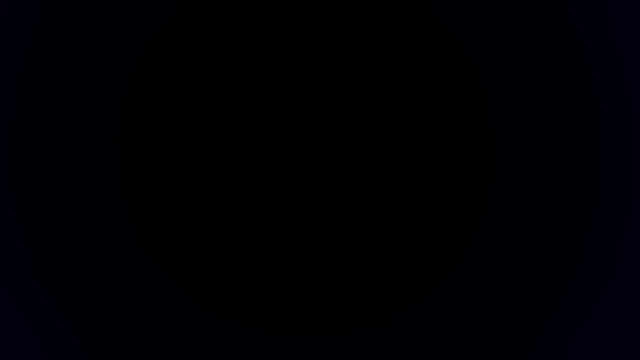 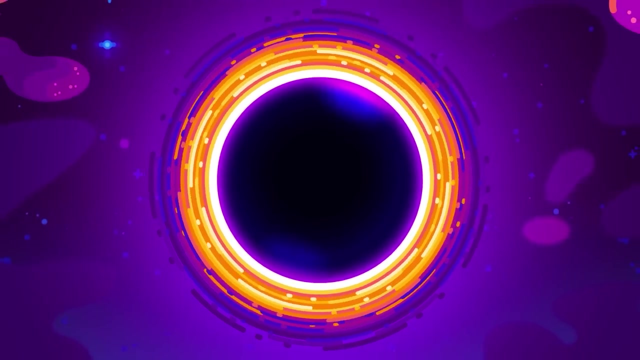 absolutely nothing can escape from its surroundings, not even light. This is why a black hole looks like a black sphere of nothingness. The event horizon is the outer edge of this ultimate prison. Cross it and you'll never be able to come back. But when a black hole rotates, it works a bit like 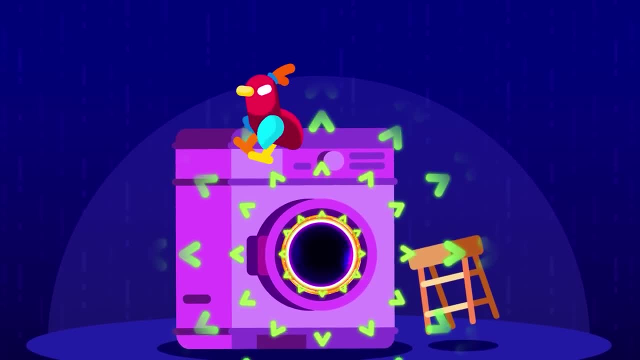 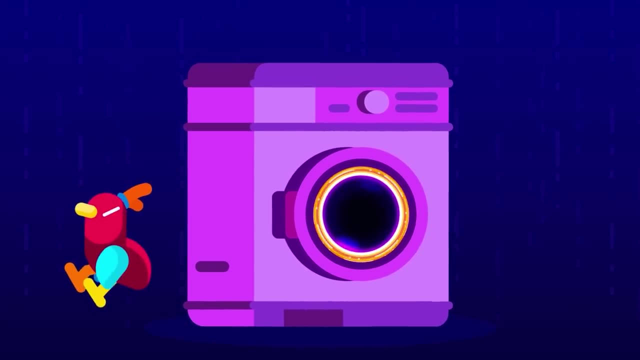 a spinning washing machine Experiment. 5. Destroy the event horizon. It's true that a black hole is as if the rotation wants to repel nearby objects and push them out of the black hole, which doesn't happen because its gravity is so strong, But if the rotation gets too fast. 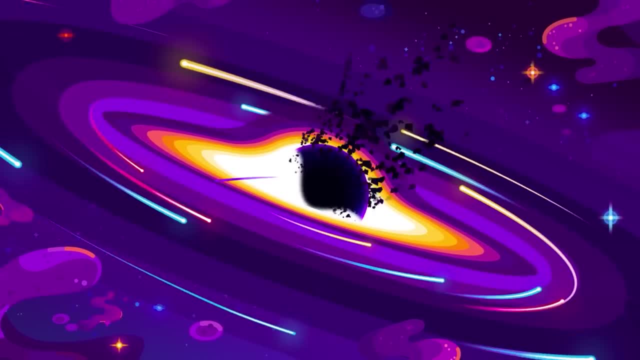 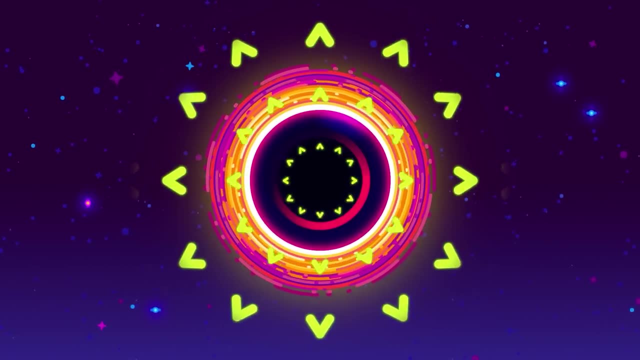 this effect will win and the event horizon will disappear. Nearby objects won't be imprisoned forever anymore. The same thing happens with the electric charge. Make it too large and our ironclad jail will break open. If we manage to destroy the event horizon, the singularity would. 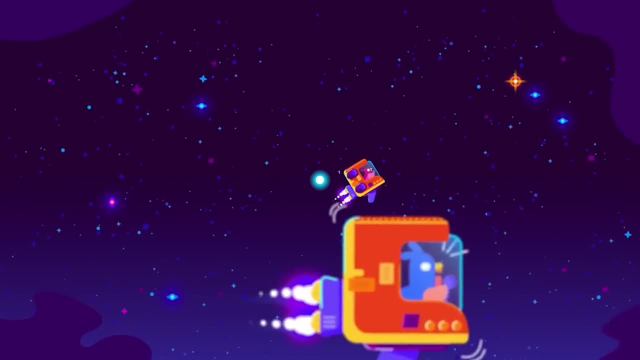 still be there and objects would still naturally fall to the ground. But if we destroy the event horizon, the singularity would still be there and objects would still naturally fall to the ground. If you hit it, you would still die horribly and quickly, But the vicinity of the singularity 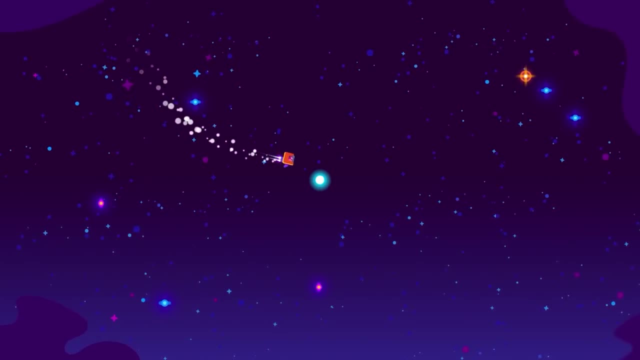 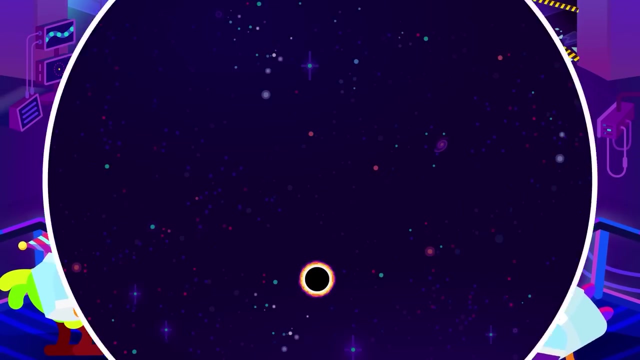 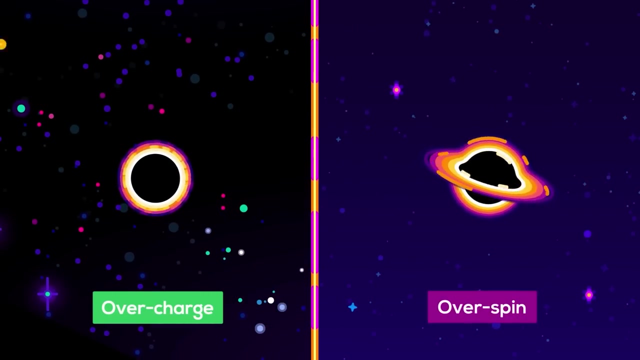 won't be an inescapable prison anymore. You could get as close as you want and come back. This should count as destroying the black hole. Can we do it? Experiment 5. Overfeeding: All we have to do is to overcharge or overspin the black hole. 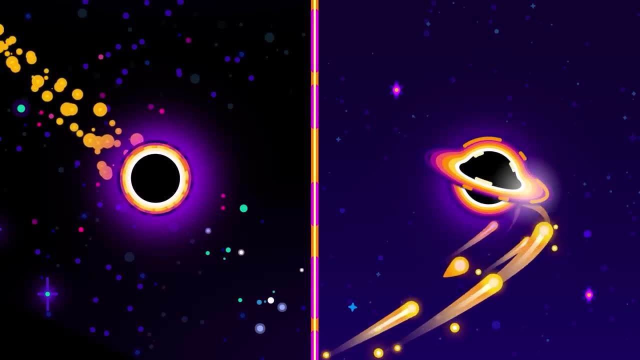 We could do this by throwing objects with a small mass and a lot of charge or angular momentum, so that the charge or spin in the black hole would be the same as the charge in the black hole And an excess charge increases faster than the mass. We have to overfeed the black hole until it. 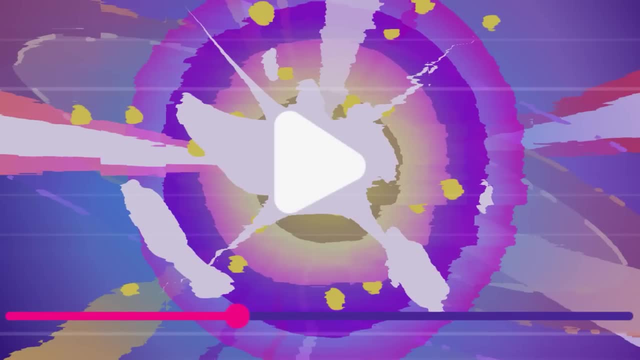 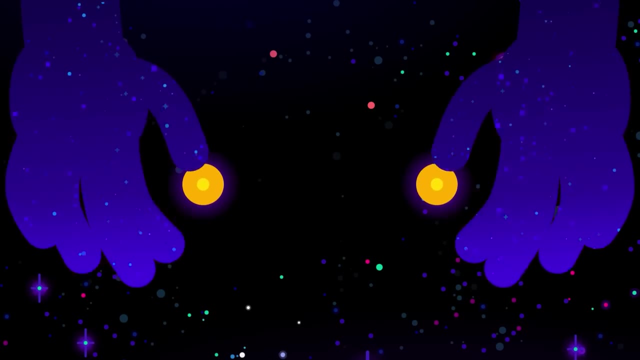 reaches the point where it breaks open. However, whether you can actually do this is the subject of passionate argument among physicists. Think of a charged black hole. Equal charges repel each other, and the more of the same charges you squish together, the more they push back. So let's say: 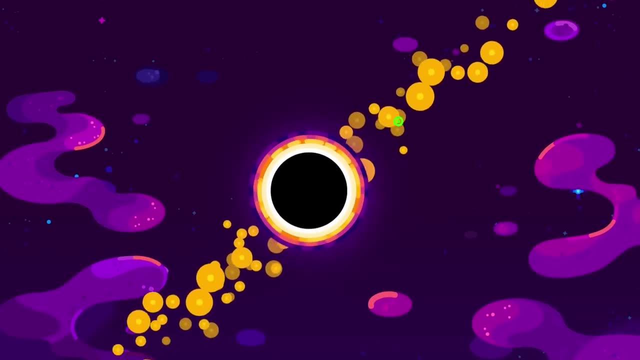 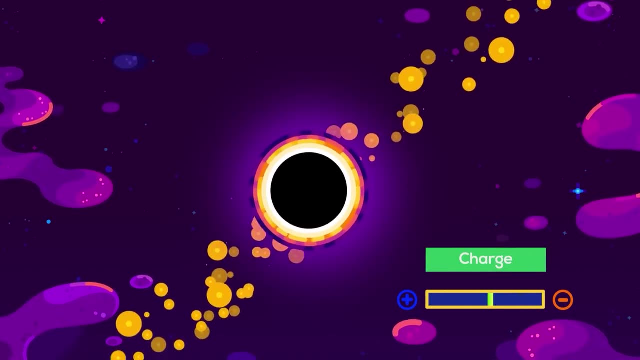 that we have a negatively charged black hole and we want to overfeed it with electrons, for example, whose charge is far larger than its mass. The electrons will feel an electrostatic repulsion And the more electrons we throw, the larger the negative charge of the black hole will be and the stronger the repulsion. 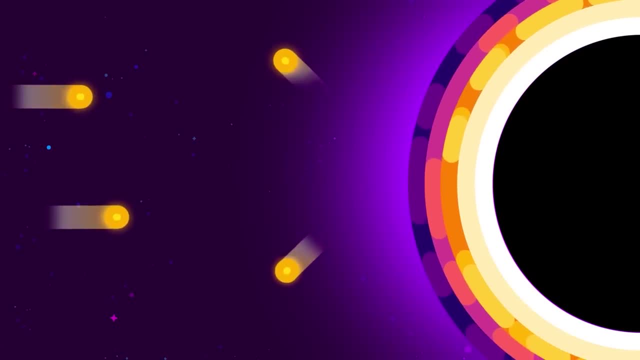 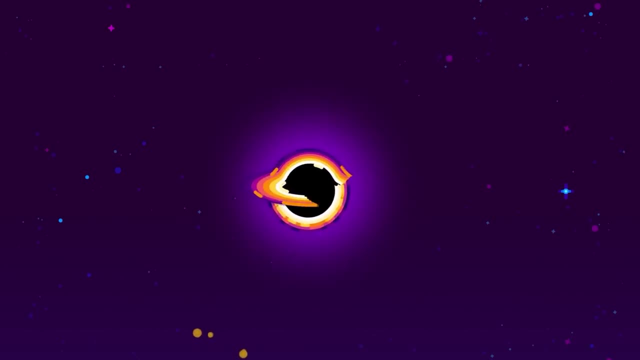 But once we reach the upper limit, the electrostatic repulsion will be so strong that it won't allow any more electrons to come in. At this point the black hole will refuse to be overfed With the spin. it's similar. 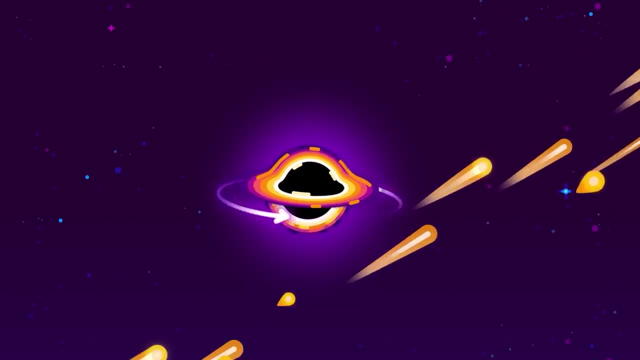 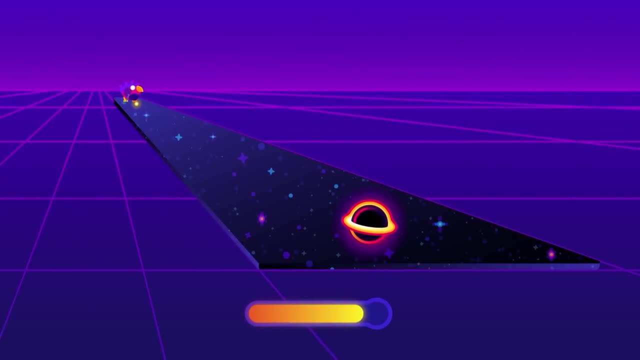 Once the black hole reaches its upper limit, it won't gobble more spin. But some scientists have discovered what looks like a loophole. If, an instant before the black hole reaches the limit, we throw the right amount of matter in in just the right way, it looks like we could actually overfeed it. 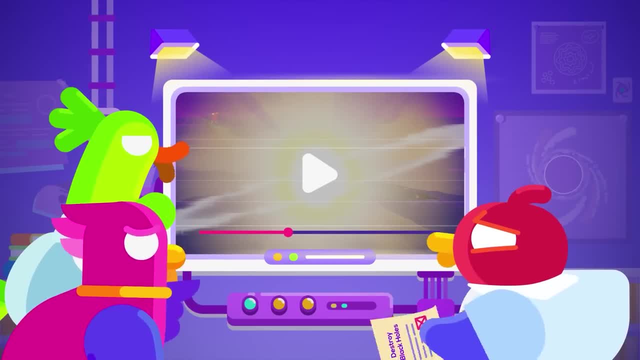 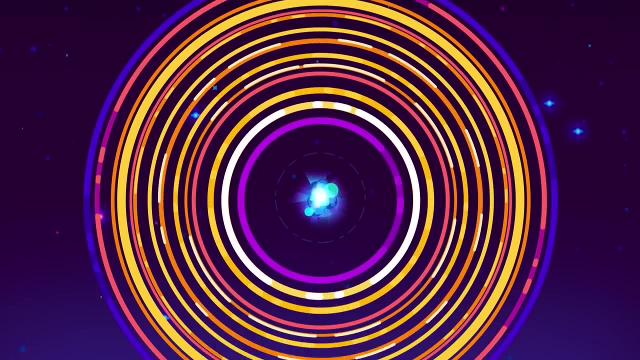 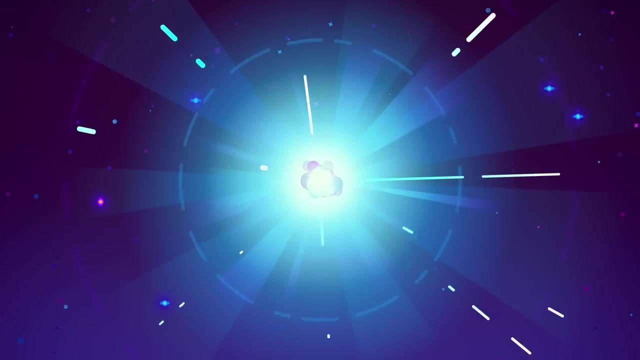 Most scientists are skeptical, but let's give it a try anyway. The end Breaking physics. There is a catch, though: The event horizon of a black hole hides the singularity, So destroying the horizon would leave us with a naked singularity, one that is not hidden by an event horizon. 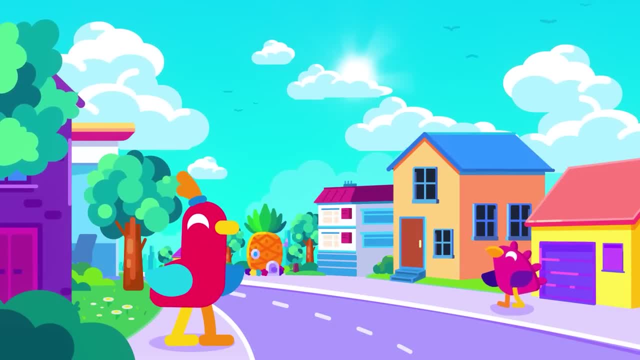 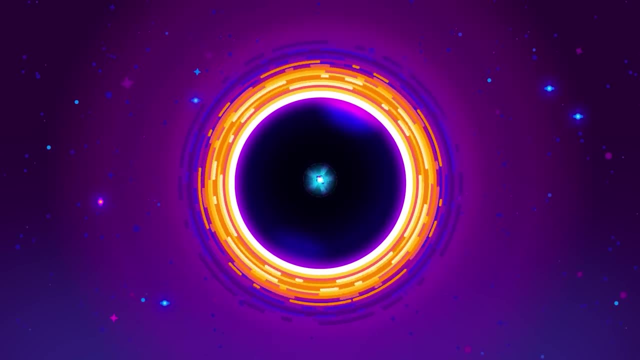 And this poses a problem. It could mean the end of physics as we know it. There's a big, dirty secret about black holes. Contrary to widespread belief, the singularity of a black hole is not really at its center. No, it's in the future of whatever crosses the horizon. 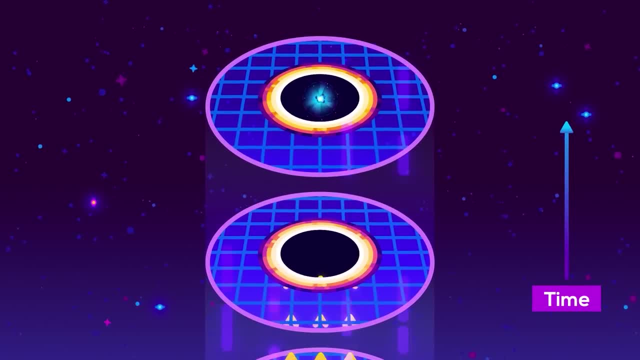 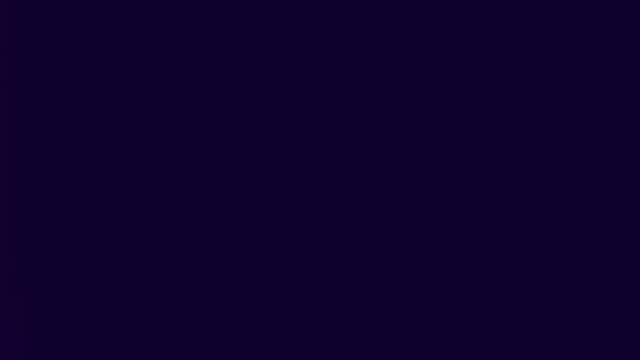 Black holes warp the universe so drastically that, at the event horizon, space and time switch their roles. Once you cross it, falling towards the center means going towards the future. That's why you can't escape. Stopping you from escaping is a problem. 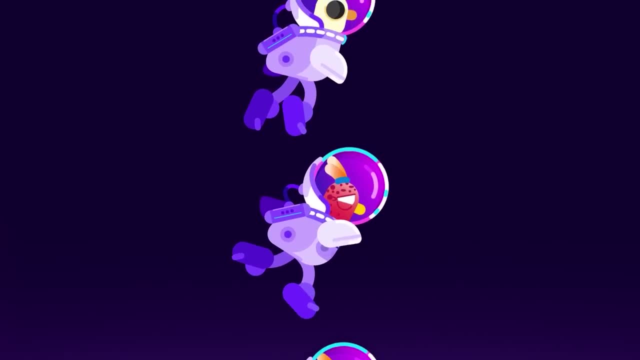 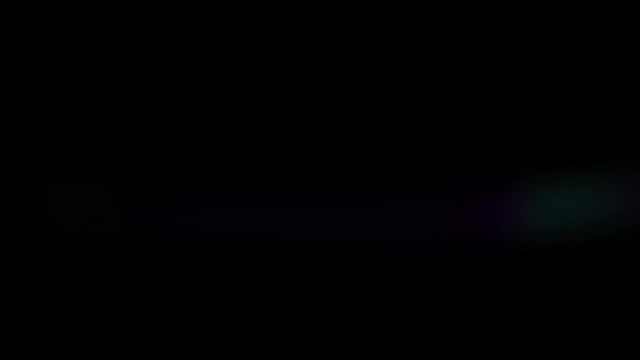 And turning your fall and turning back would be just as impossible as stopping time and traveling to the past. So the singularity is actually in your future, not in front of you. And just like you can't see your own future, you won't see the singularity until you hit it. But you also can't hit something that's in your future. only sort of experience it, Like you'll experience your next birthday, when it happens. Singularities that are in the future are not a problem because we can't see them or interact with them. But a naked singularity would be in front of you. But a naked singularity would be in front of you. But a naked singularity would be in front of you. But a naked singularity would be in front of us for all of us to see. 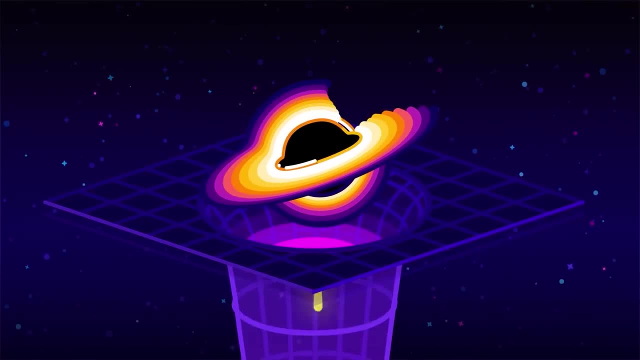 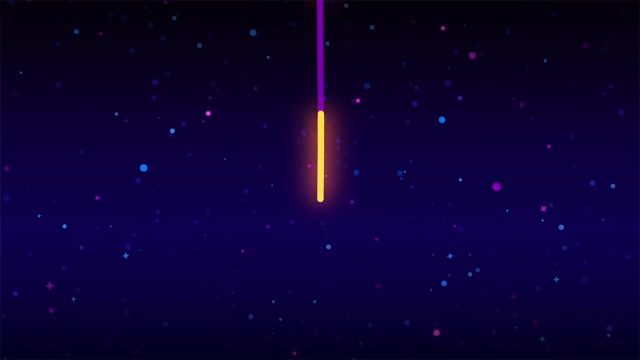 What would we see? Well, the whole point is that it's impossible to know. A singularity is a region of infinite gravity, and gravity is the bending of space time. At a singularity, the bending is so radical that the fabric of space time is literally broken. 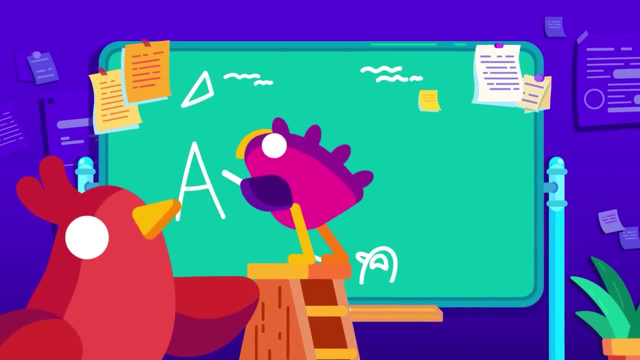 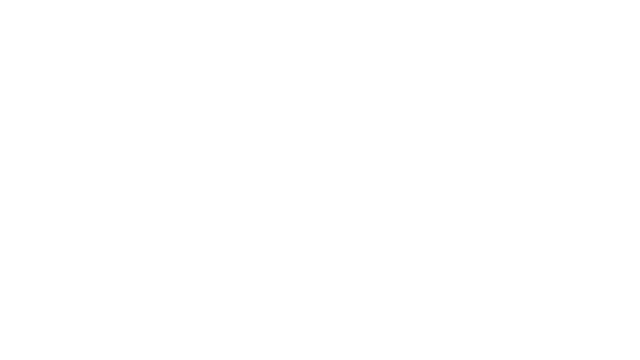 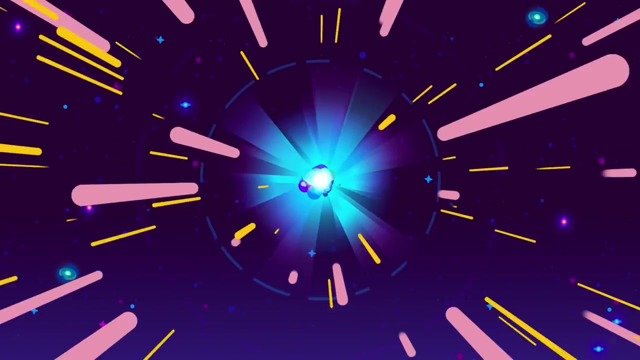 Space and time don't exist anymore. This means that you can't predict anything, since predicting means making a forecast about where and when something will happen and when have lost their meaning. So we have an unpredictable thing with infinite gravity and therefore infinite energy. 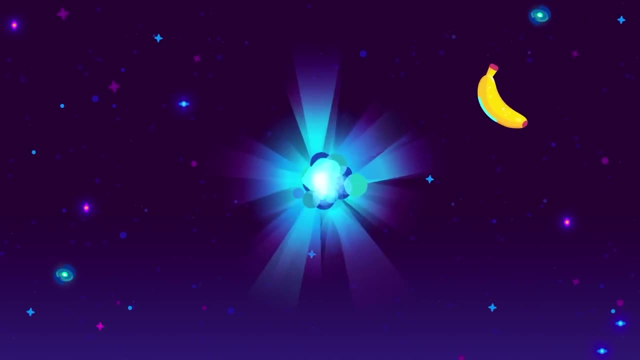 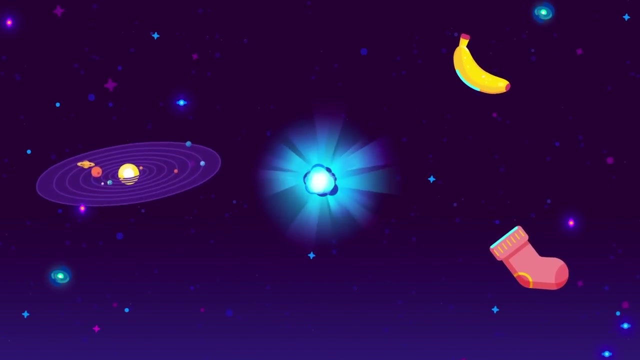 This means that anything could come out of it for no reason, from a pile of bananas to lost socks or a solar system. Predictability, causality and physics as we know it would break down. We think that singularities should exist in nature. 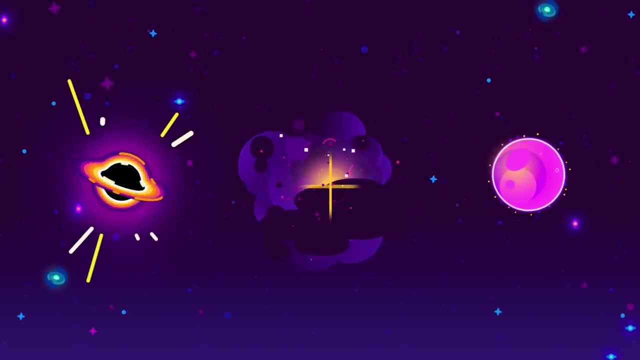 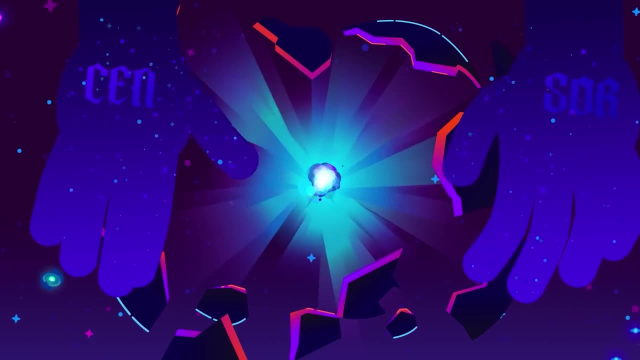 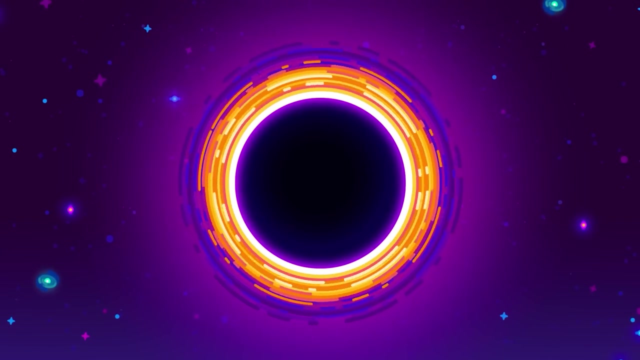 because we can prove that, under very general conditions, gravitational collapse leads to the formation of singularities. However, scientists think that nature forbids the formation of naked singularities. Something enforces the creation of an event horizon around them to prevent their insanity from infecting the rest of the universe. 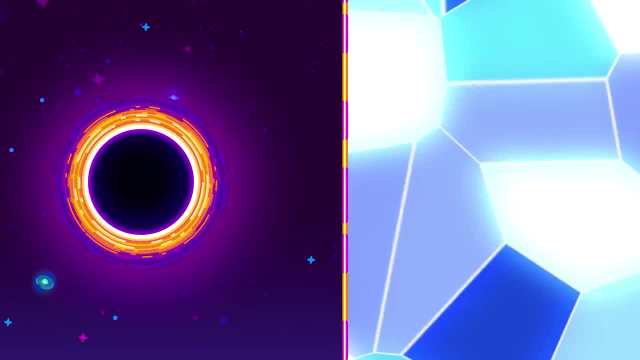 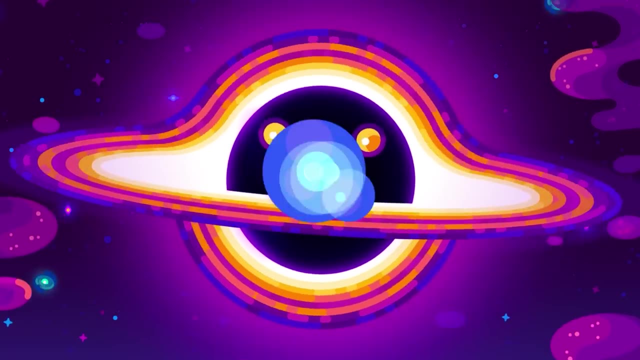 Without event horizons, physics may not make sense at all. So although black holes have been portrayed as the ultimate monsters of the universe, they may actually be the heroes that keep us safe from the madness of singularities. So if we do destroy the horizon, 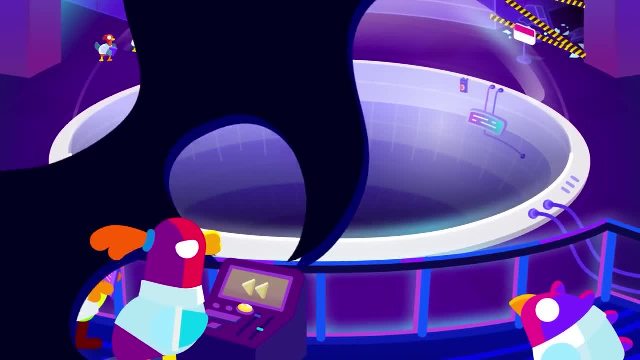 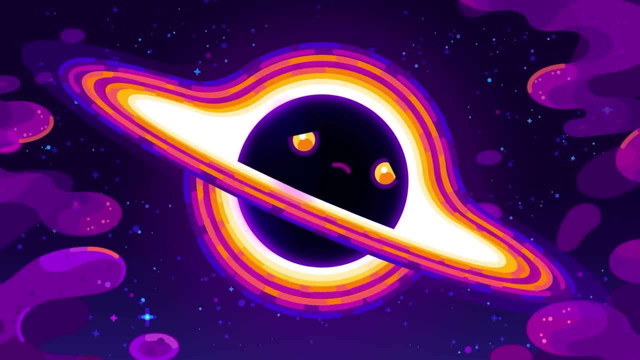 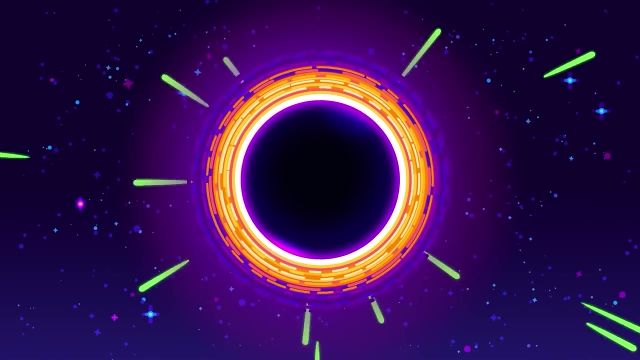 we might destroy the fundamental rules of the universe. You know what? Let's not do that. Conclusion: the safe option. As far as we know, there's just one safe method to destroy a black hole weight: All black holes emit tiny particles. 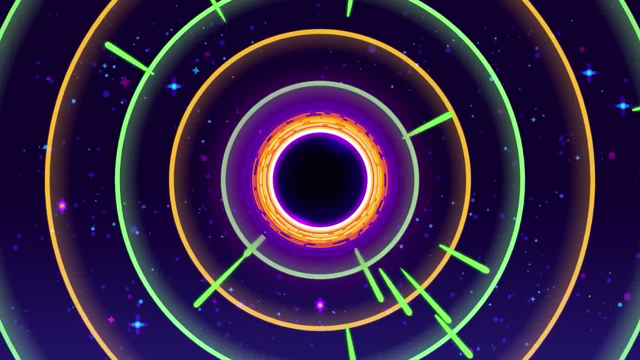 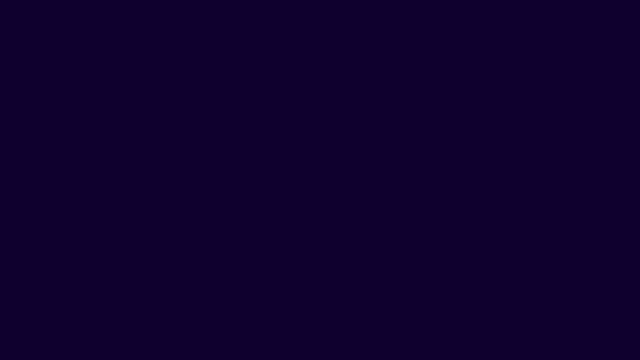 a phenomenon called Hawking radiation. This process causes them to slowly lose mass until they eventually evaporate, leaving behind no horizon and no naked singularity. The time it takes for a black hole to completely evaporate depends on its mass. For our mini black hole, 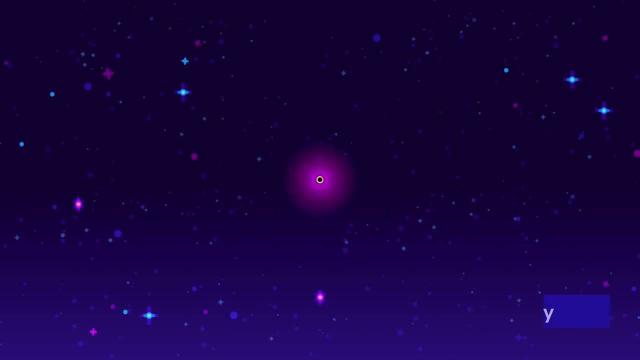 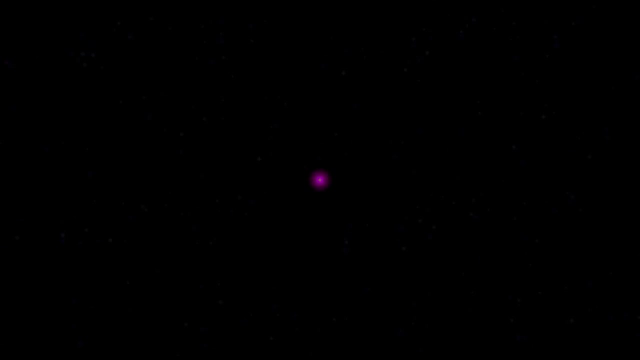 the science of a specific black hole. it will be about 10 to the power of 44 years, 10 billion trillion trillion times the present age of the universe. So is it possible to destroy a black hole? Yes, we just have to wait. 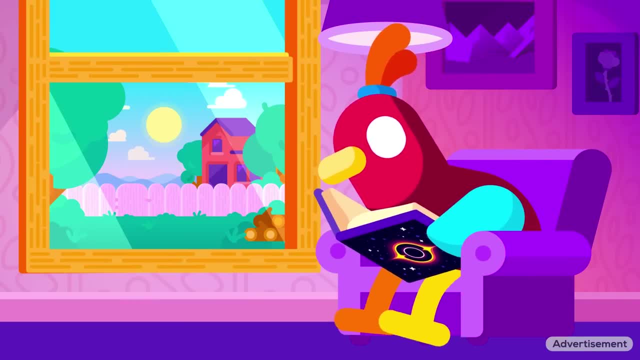 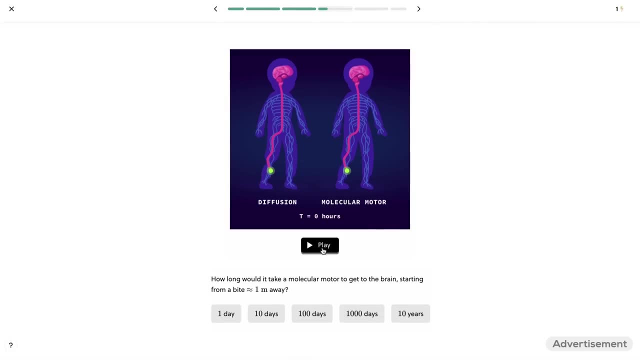 But you don't have to wait that long. There are plenty of fascinating things to explore right here on this planet right now, if you have the knowledge to understand them. To help you with that, we've created a series of lessons to take your scientific knowledge to the next level. 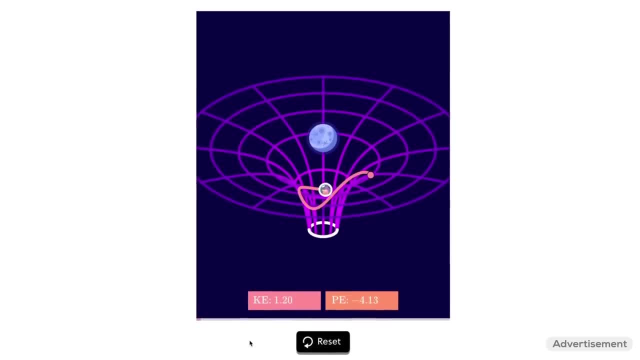 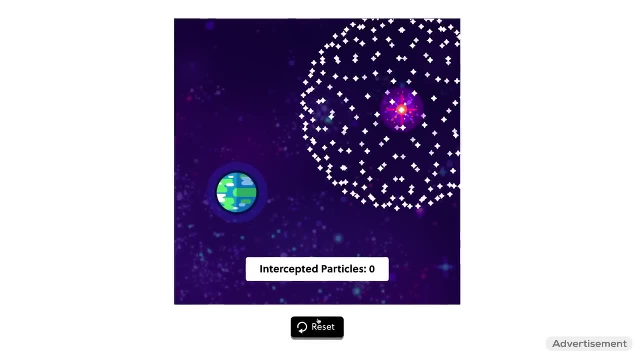 made in collaboration with our friends at Brilliantorg. These lessons give you a deeper understanding of the topics from our most popular videos, from rabies and mammalian metabolism to climate science and supernovas. There's even a lesson on black holes where you can delve into the fundamental principles. 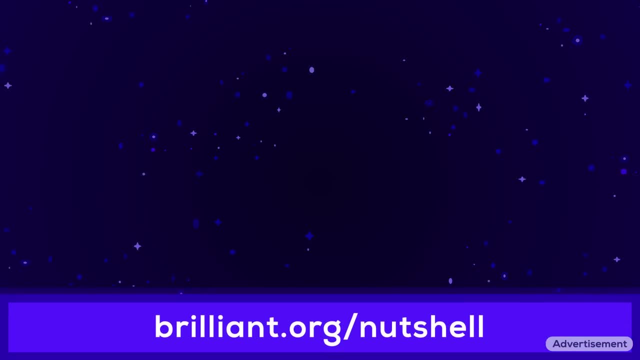 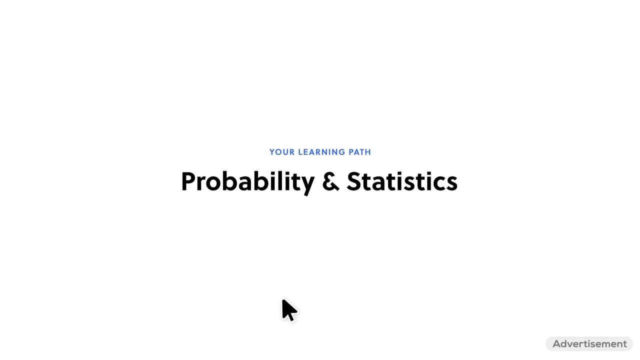 behind their behavior and life cycle. Brilliant is the best way to master key concepts in everything from maths and science to computer science and beyond. Just set your goal and Brilliant designs the perfect path and equips you with the right tools to reach it. Brilliant has thousands of lessons to explore. 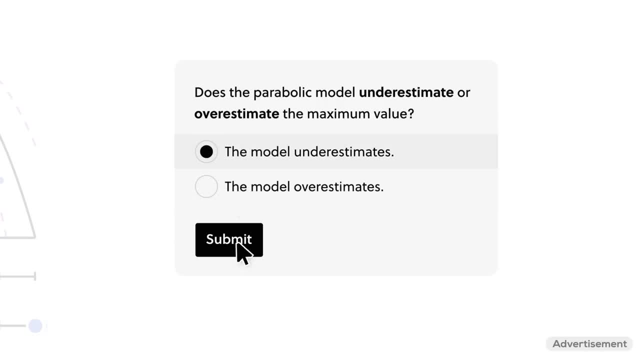 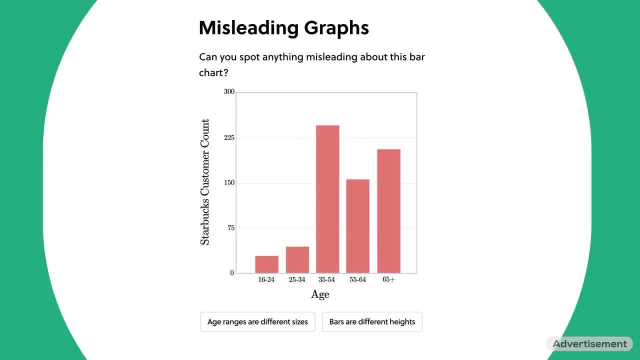 and each one is interactive like a one-on-one version of a Kurzgesagt video. Their latest course, Exploring Data Visually, will teach you everything you need and nothing you don't. to start your journey in data science, No coding skills required. 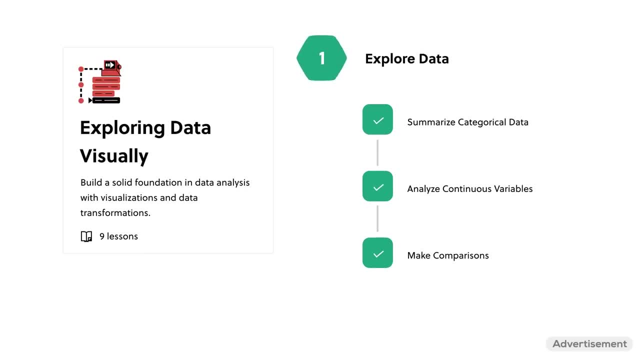 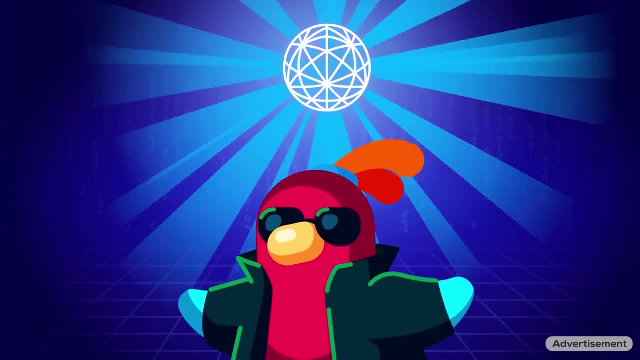 You'll analyze real data sets, like one about Starbucks, and learn the skills to draw insights for yourself. In a world overflowing with information, data skills are becoming essential in virtually every field. Brilliant is the perfect place to start learning them. To get hands-on with Kurzgesagt.